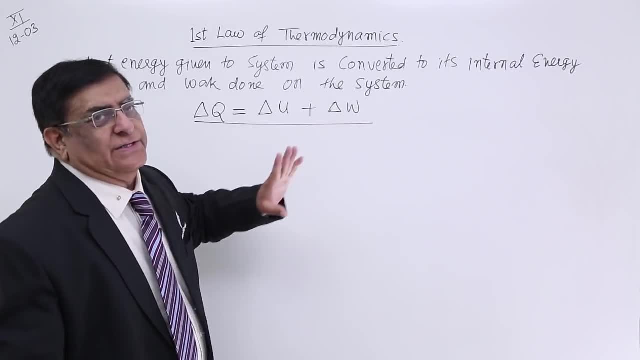 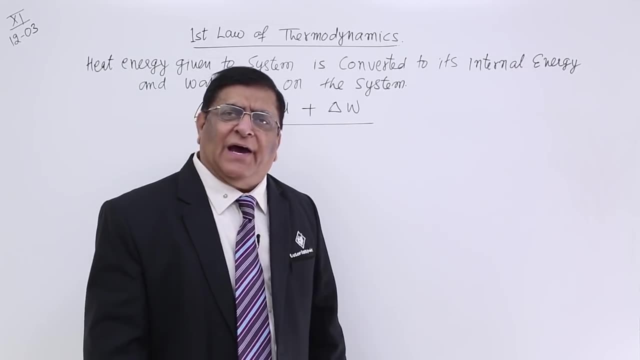 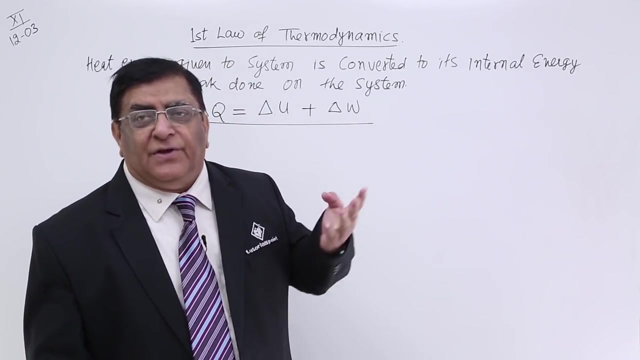 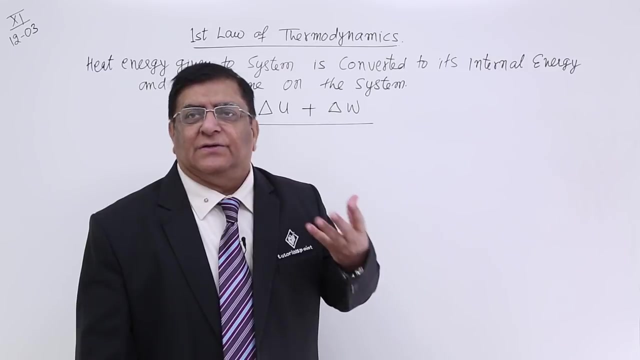 Okay, Delta W. we have to understand What is this: Work done on the gas Or work done by the gas? Either way, How can we calculate this delta? work done with the parameters of the system? We know the parameters, which are heat, energy, pressure, volume, temperature, all these 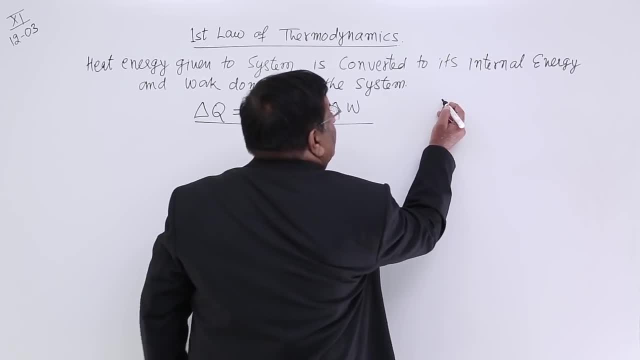 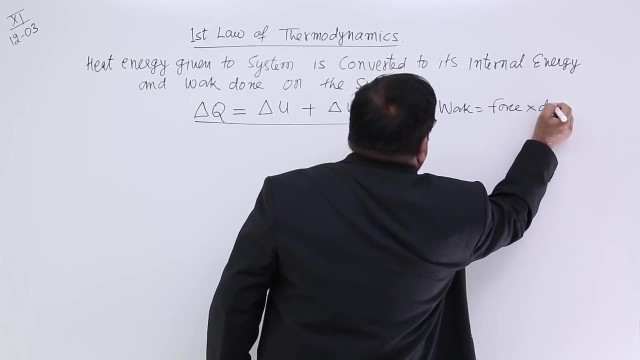 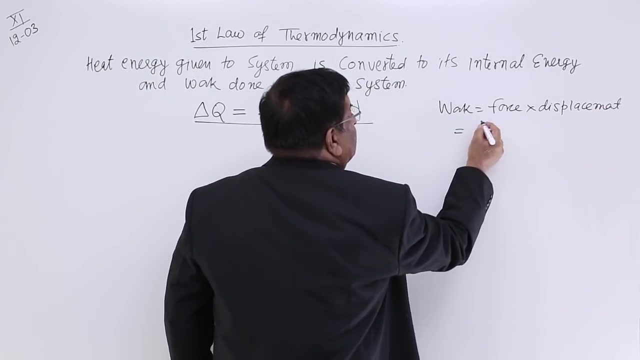 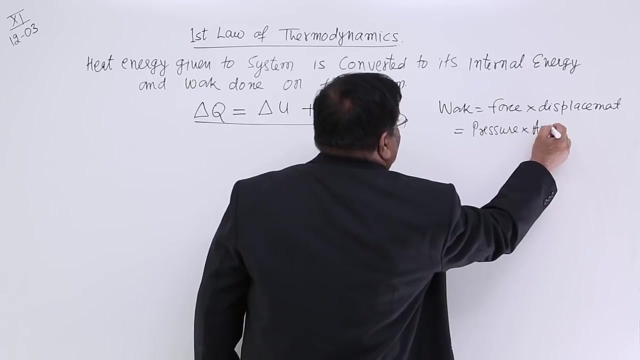 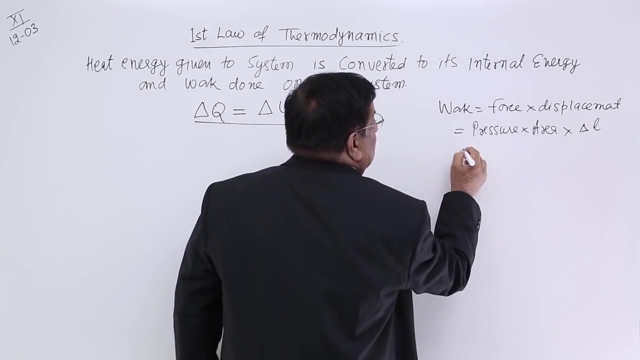 What is work done? So I tell you here a very small calculation. work is equal to Force into displacement. force in the terms of pressure can be written as pressure into area, and this is displacement, that is change in length. So this is pressure: P area into length. 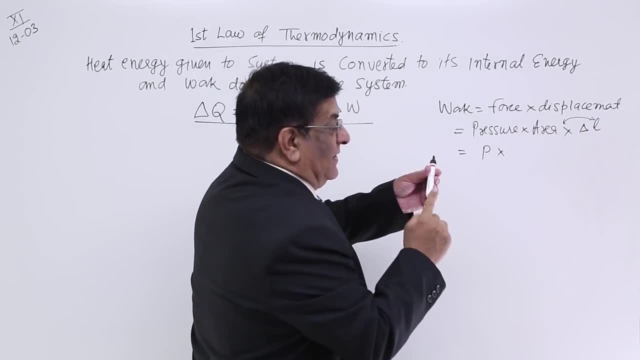 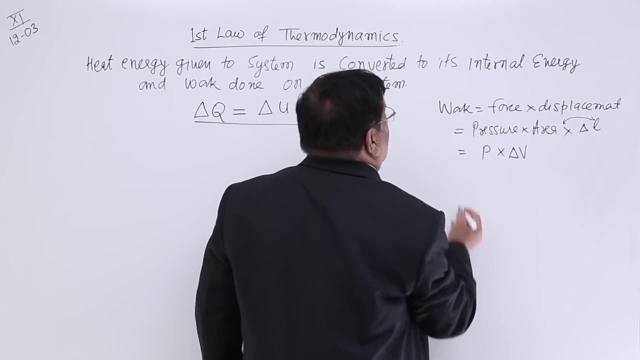 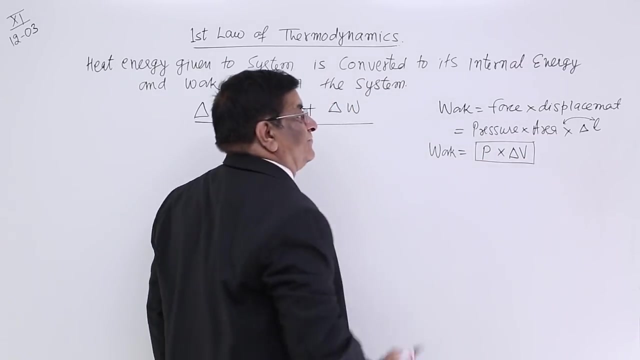 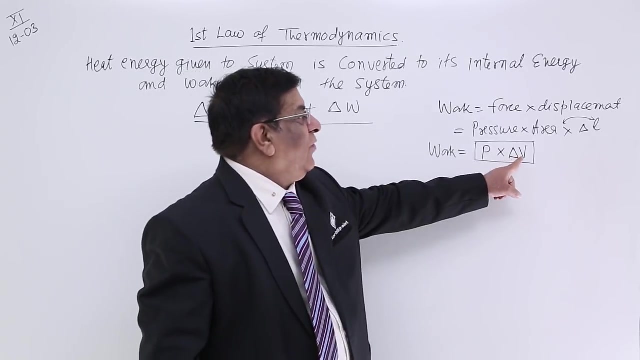 Area of displacement, Area of cylinder into length. that gives the volume. So this is delta V. So work done on the gas is given by P into delta V. Okay, If the total energy we want to calculate the total energy is the total volume. 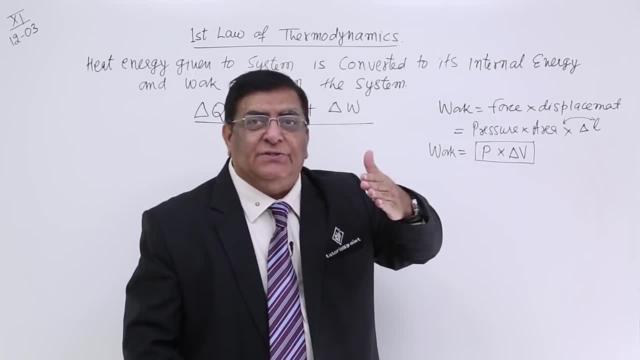 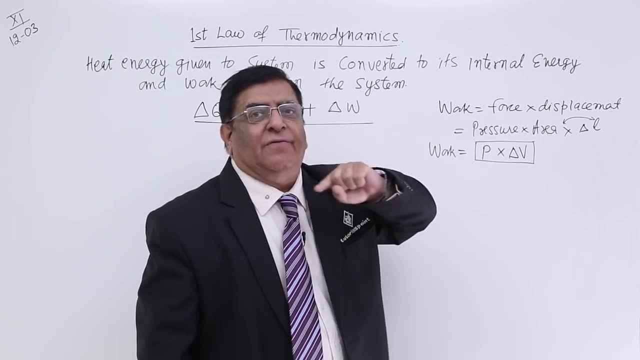 Delta V shows what How much fresh work has been done. Already there was certain energy. It was having energy of 1000 joule. We have done a work of 200 joule. Now it has become 1200 joule. 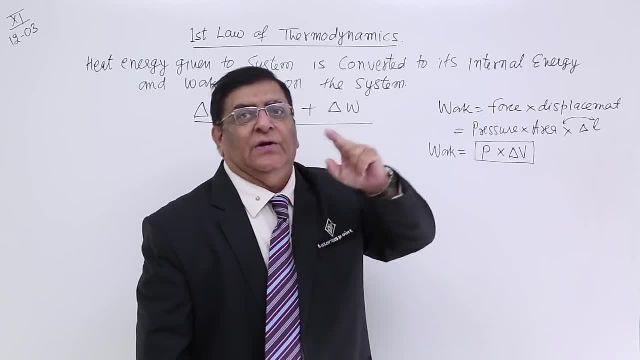 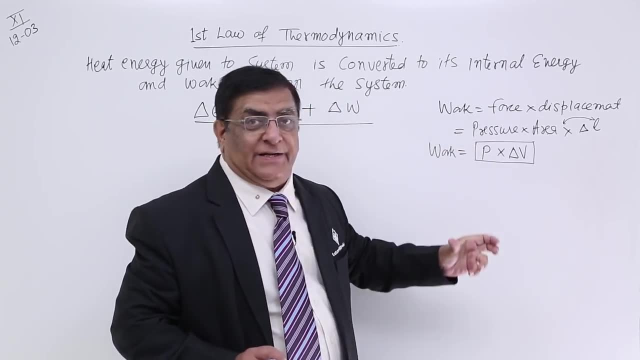 So P delta V is doing the calculation of the 200 joule. What work we have done. and because of that work that piston has moved In the cylinder, So that is change in volume. So work will be given by pressure into delta V. 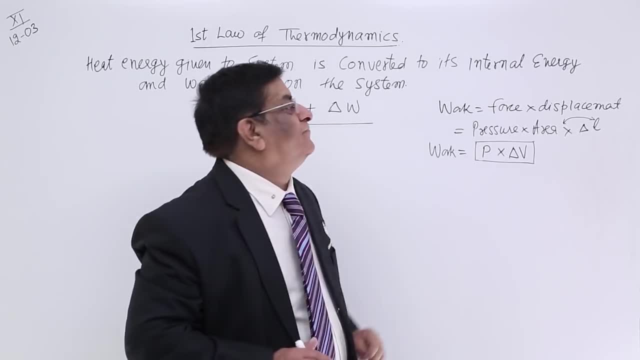 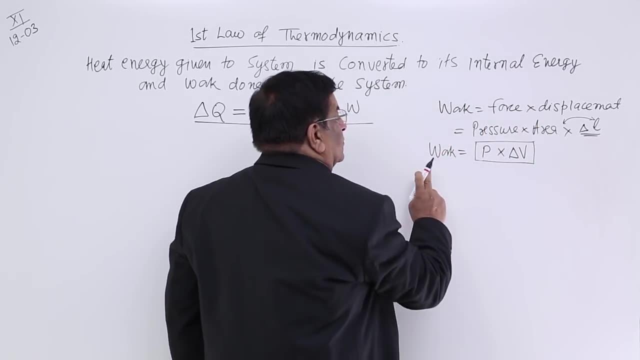 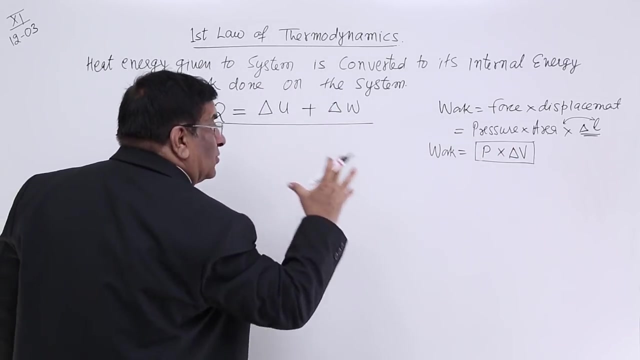 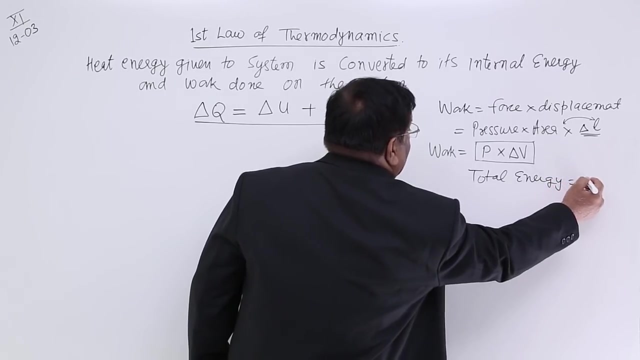 Change in volume, Because there was a change in volume, Because there was a change in volume, Because there was a change in length here In our calculation. So work will be small. work will be given by P into delta V. The total energy when we need we will use. total energy of the gas is P into total volume. 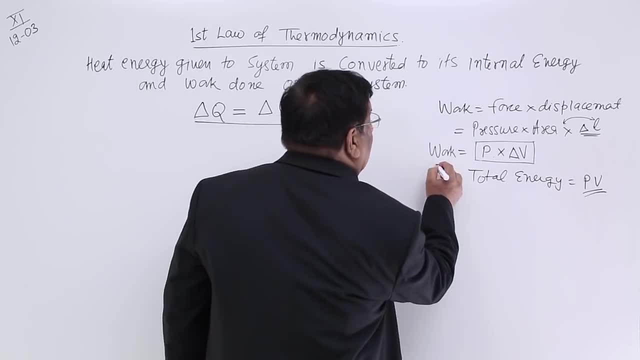 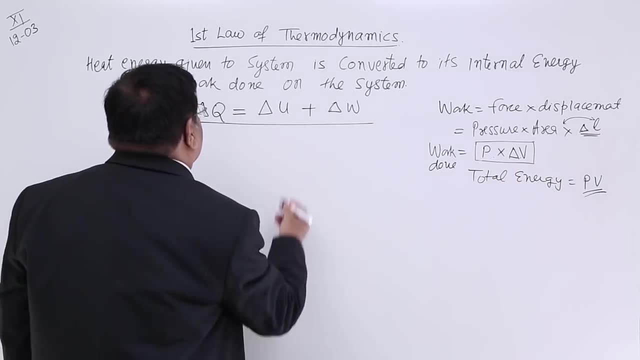 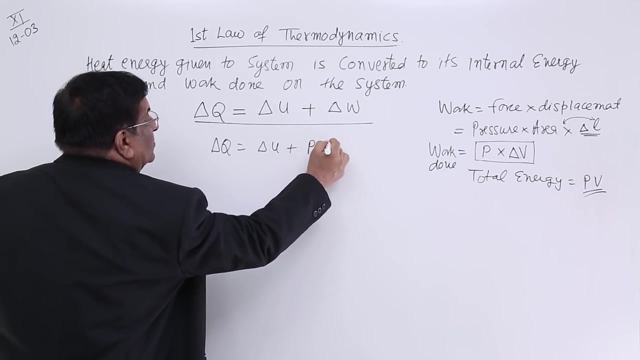 PV. PV is the total energy and work done for a small change, For a small displacement, Is given by P into delta V. So now this equation can be rewritten as delta Q is equal to delta U plus P into delta V. And what is this? we know. 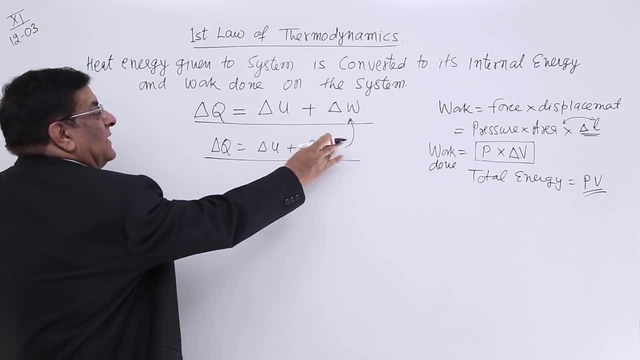 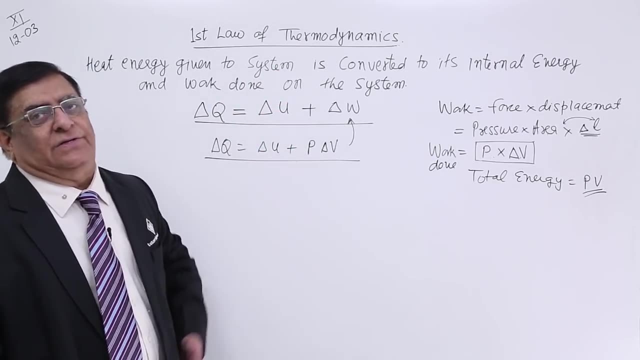 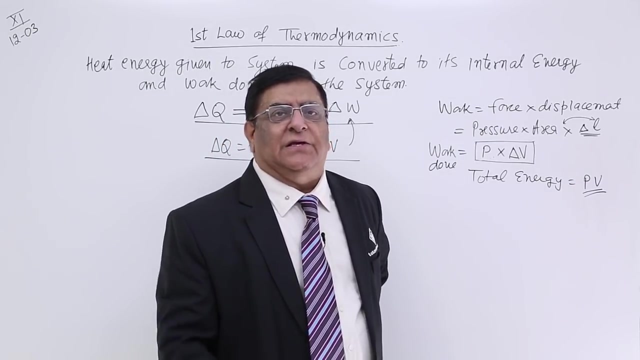 Work done, Work done on the gas or work done by the gas. Ok, So this is first law of thermodynamic. This is how it is divided. Now we can have a small example of this: We are giving heat energy to water. 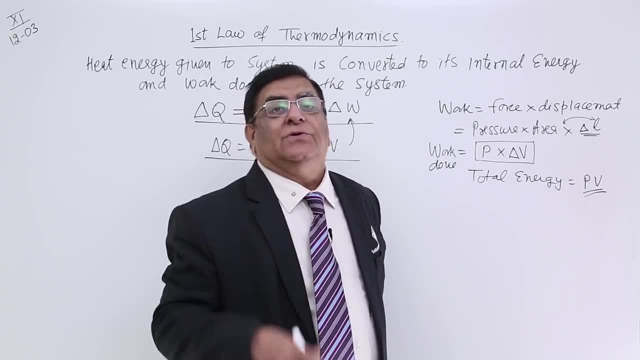 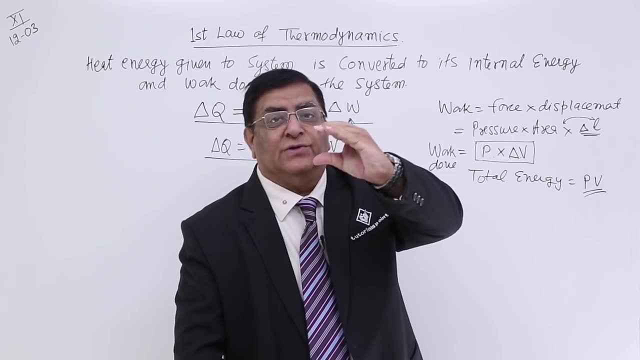 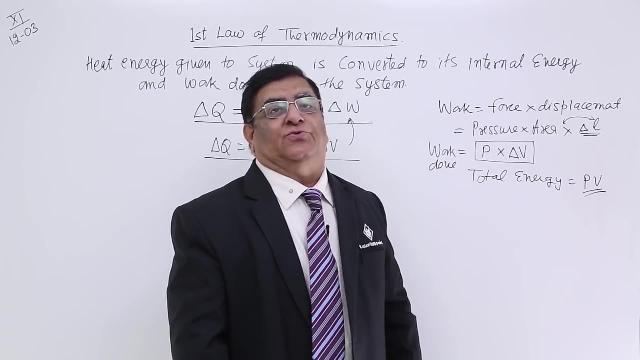 And it converts to gas. Ok, So when it converts to gas, Its volume also increase. When the volume is increased, Some work is done on the system. Who gives energy to do that work? Answer: we are heating it, So that heat gives the energy. 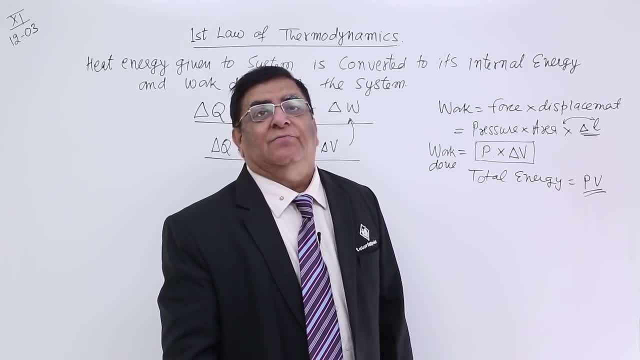 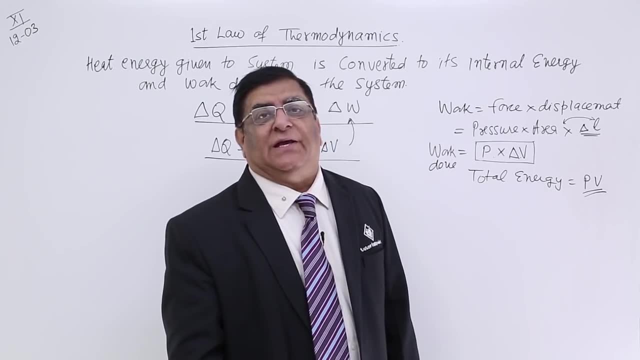 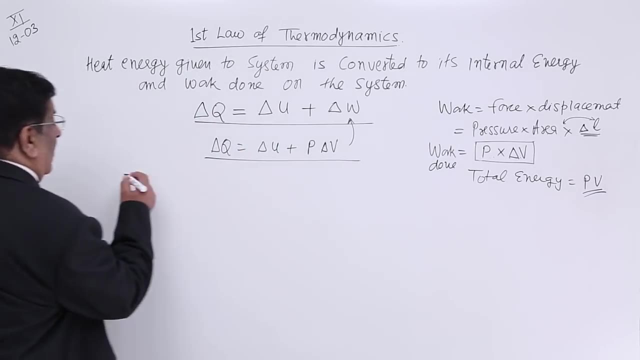 Ok, We have calculated heat By latent heat method. We have calculated how much heat is given, So we have found That we have to give it a heat of 2256 Joules. That is latent heat. Or we can say: 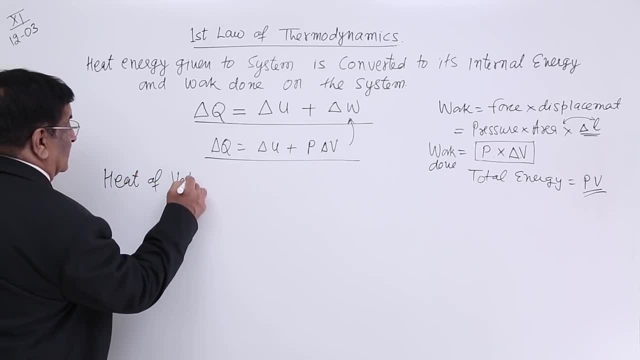 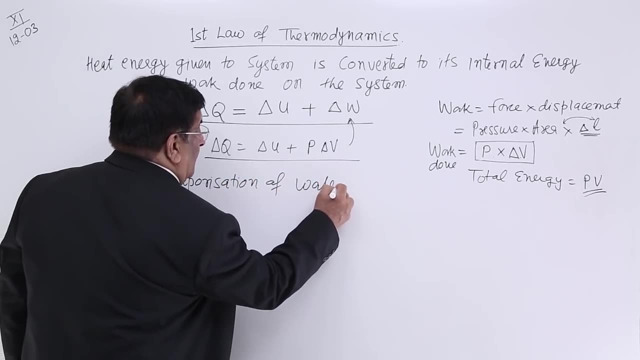 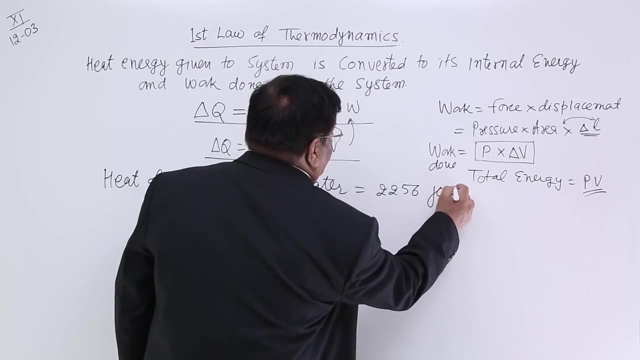 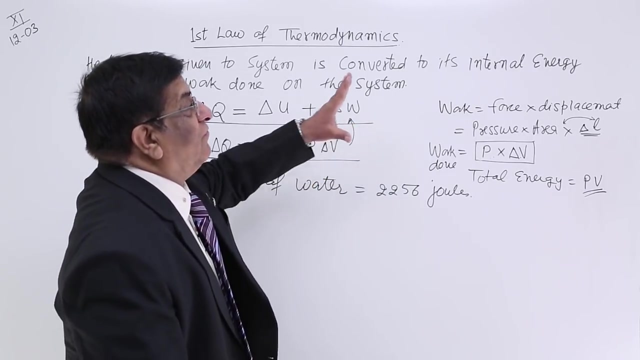 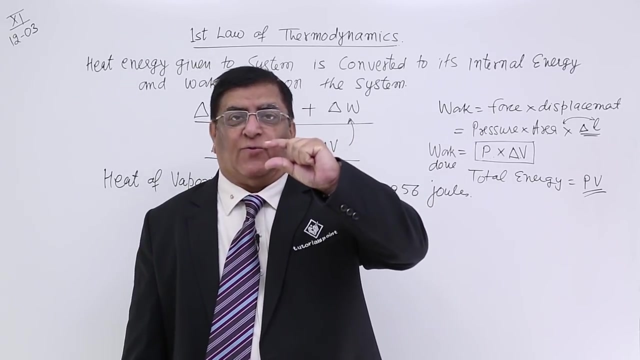 It is heat of vaporization. Heat of vaporization of water Is 2256 Joules. Ok, Now There is a change in volume. How much is change in volume? We have seen That if we take one cubic centimeter of water. 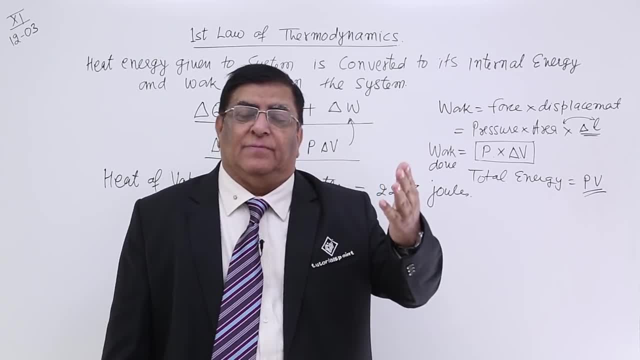 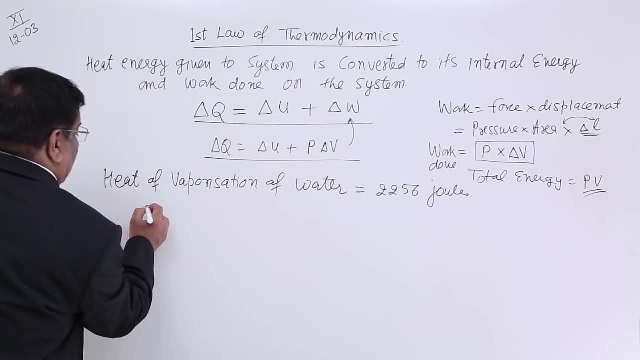 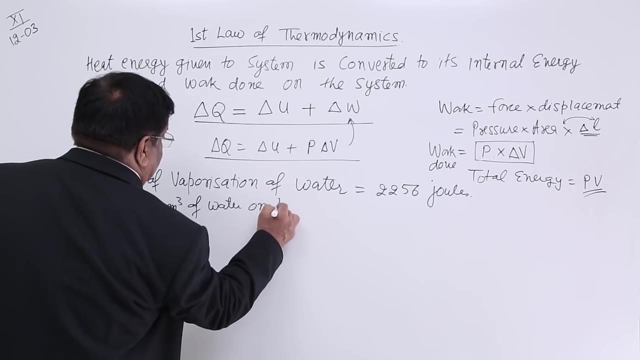 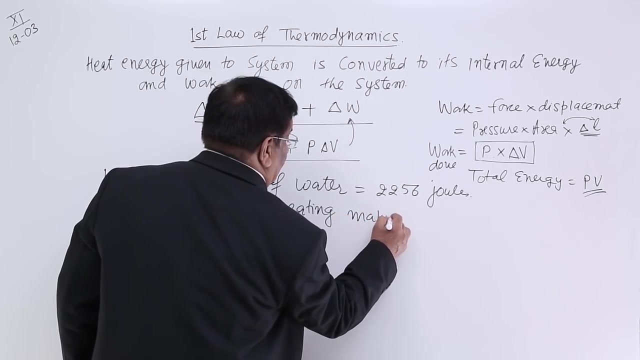 And heat. it converted into steam At normal pressure. At normal pressure That steam has a volume Equal to- I will write it: One centimeter cube Of water On heating. On heating Makes Steam Equal to. And the volume of that 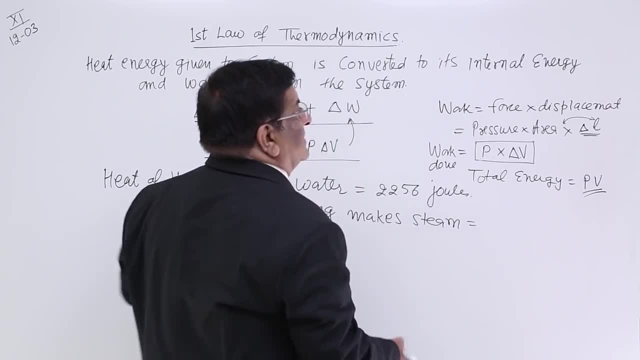 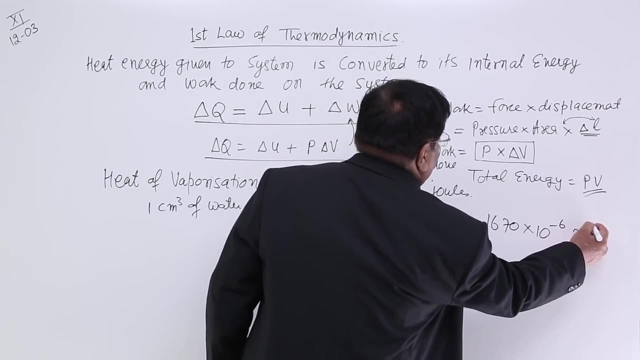 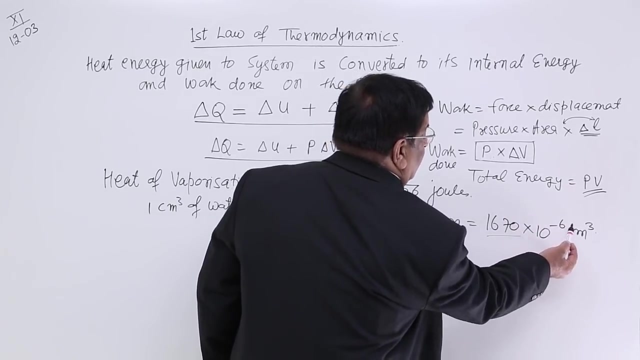 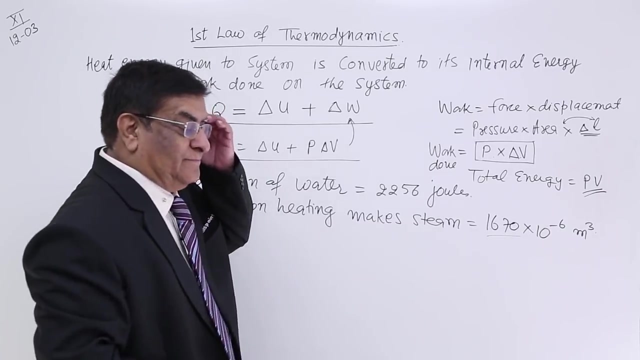 Steam Is equal to 1670. Into Power Minus 6. Meter cube, This is 1670. Centimeter cube. We convert it into meter cube. So This is the Volume. Ok, This is the change in volume. 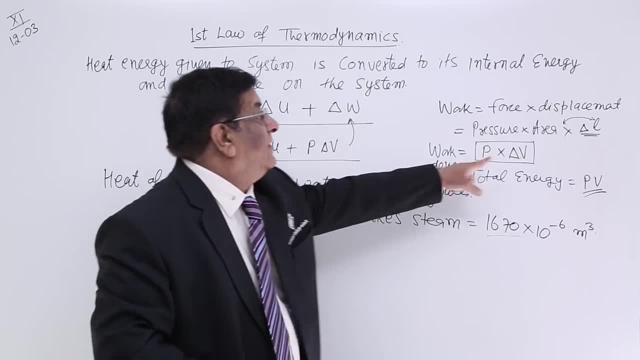 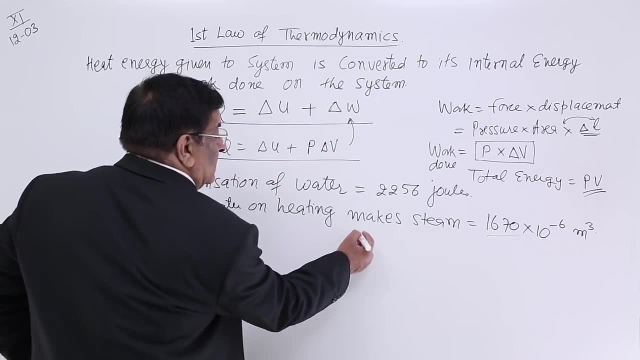 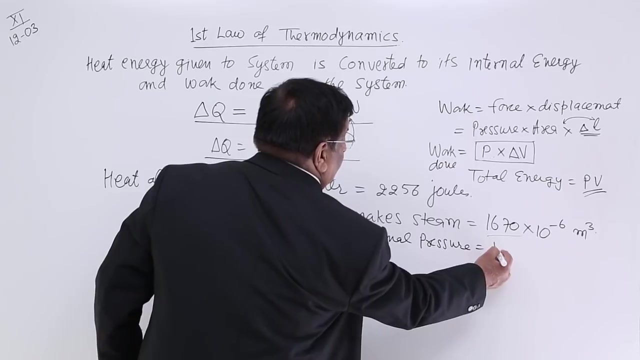 From one centimeter to This much. This is what Change in volume. How much is the normal pressure Where we have changed the volume? Normal pressure? Normal pressure is atmospheric pressure And we know the value of atmospheric pressure, That is 1.013.. 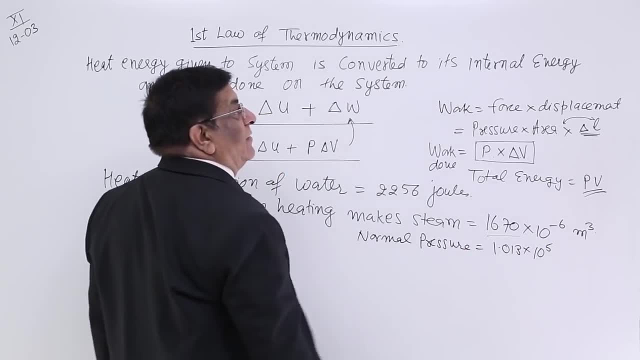 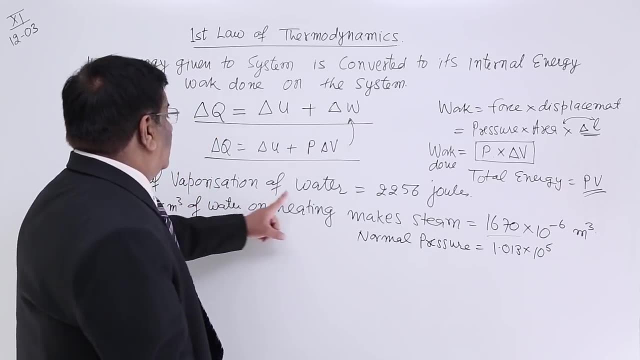 Into 10, to the power 5 pascal, Ok- Or Newton per meter square. This is normal pressure. Now, All the heat Which we have consumed Is 2256.. And we set up this equation To find out. 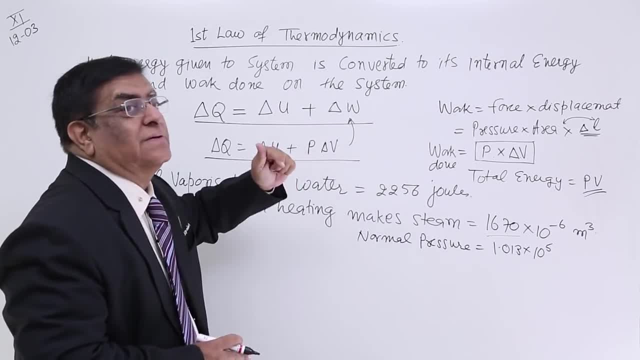 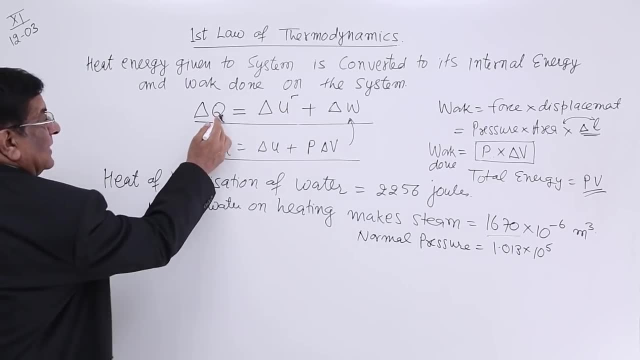 How much is the heat Given As Internal energy To this water? We want to find out. Delta U, So Delta Q Is equal to 2256.. Is equal to Internal energy Plus Delta. 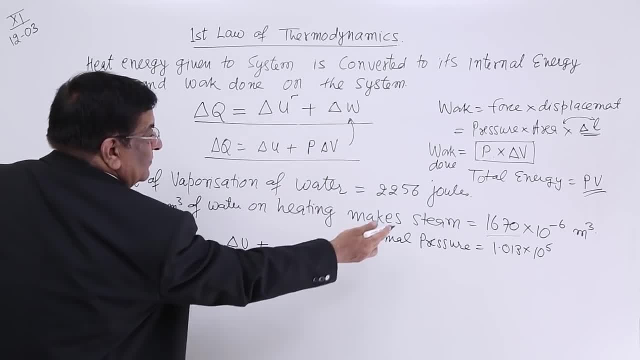 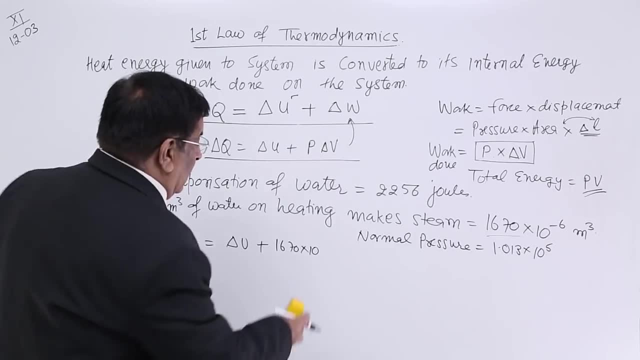 W Is P Into Delta V. P Is equal to 1670.. Into 10.. No P Is equal to this bottom one, One point 013.. Into 10 to the power. 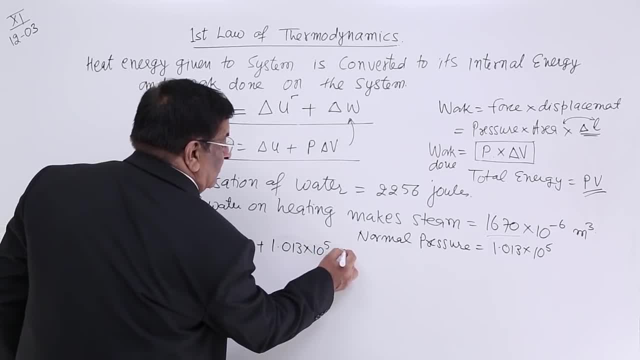 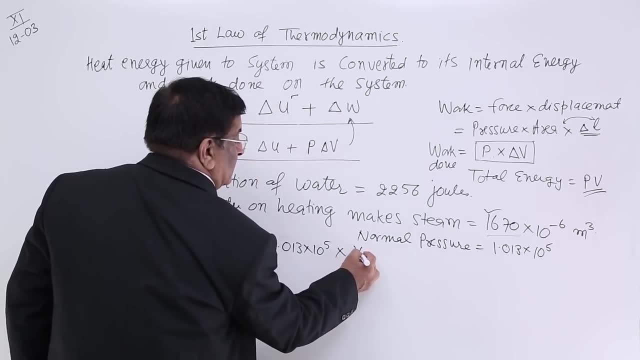 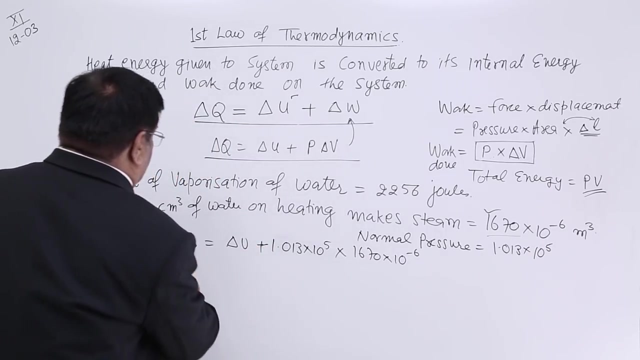 5. Multiplied By Change In Volume, The change In Volume Is This: Into 1670.. Into 10, to the power Minus 6. P Into Delta. 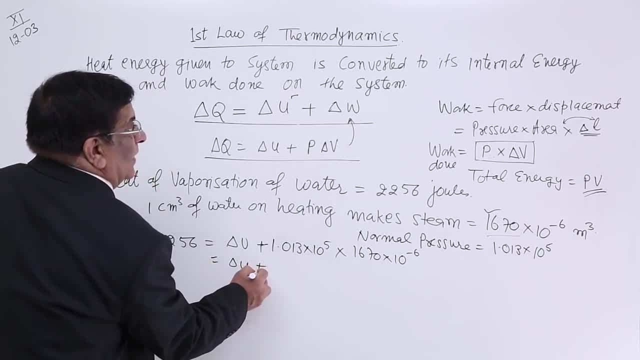 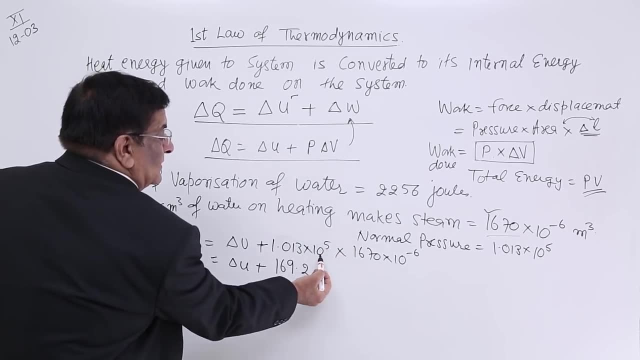 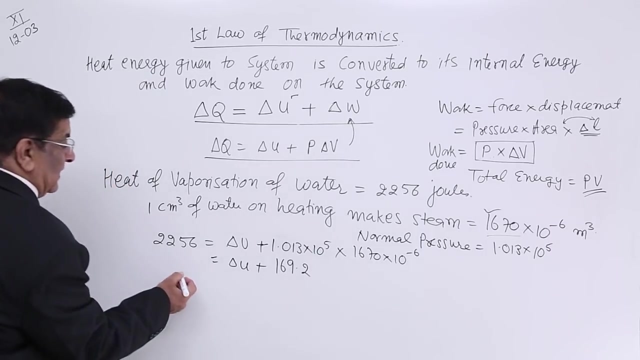 V. So This Is The Total 169.. 2. 169.. 2. This Is 10 to the power 5.. This Is Minus 6. And Multiply.